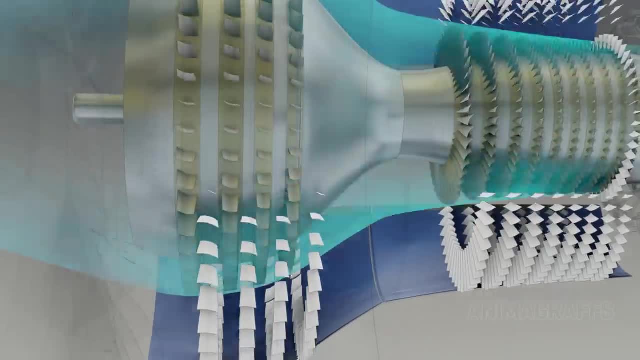 A single compressor stage is composed of a spinning rotor paired with a ring of stationary stator vanes, which likes to pump out air, from starting points to pots are attached to the core casing Rotor. blades swirl the air as they force it through the compressor. 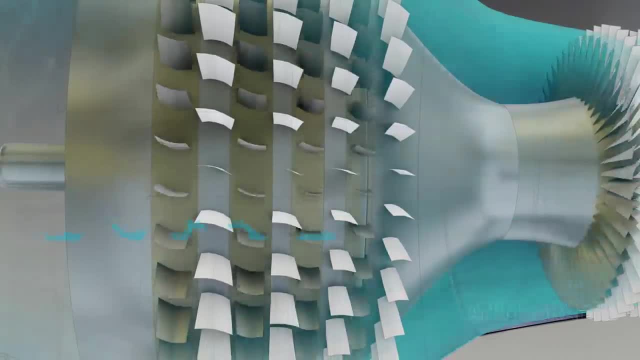 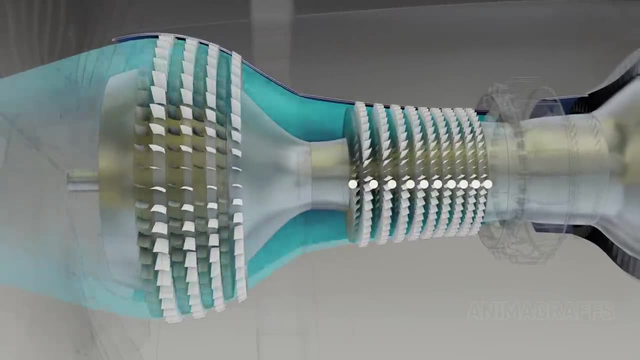 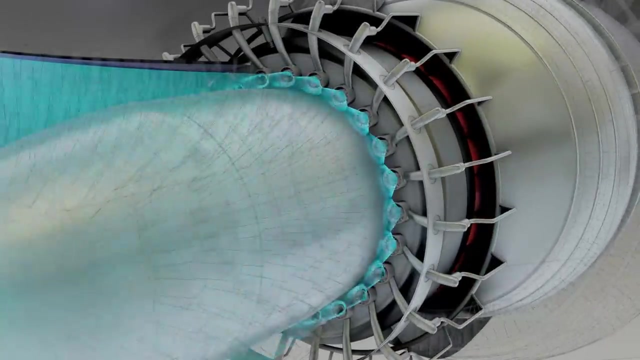 Stator vanes slow this swirling momentum in exchange for increased air pressure. The compressor has 4 low pressure and 10 high pressure stages. The Combustor Air is mixed with fuel and ignited as it passes through the combustor, releasing a jet of. 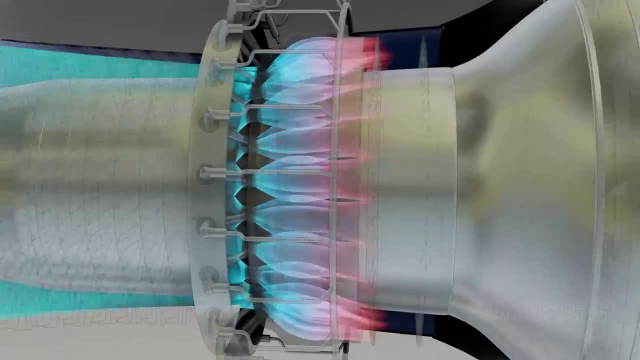 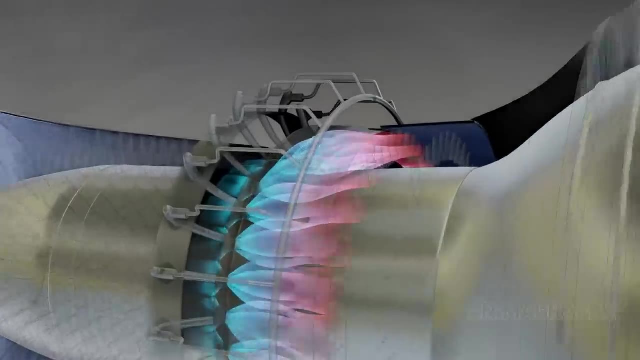 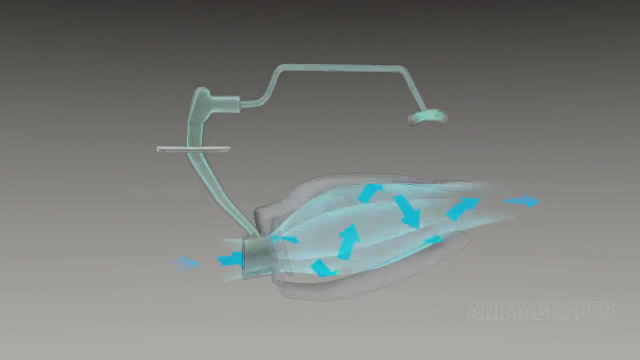 super high powered gas. The design shown here is an annular combustor, meaning ring shaped. Compressed air enters the inlet nozzles. Each nozzle is coupled with a fuel injector and is designed to swirl the incoming fuel and air for an even mix. 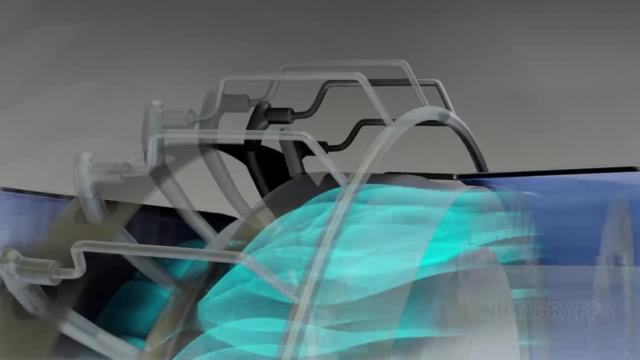 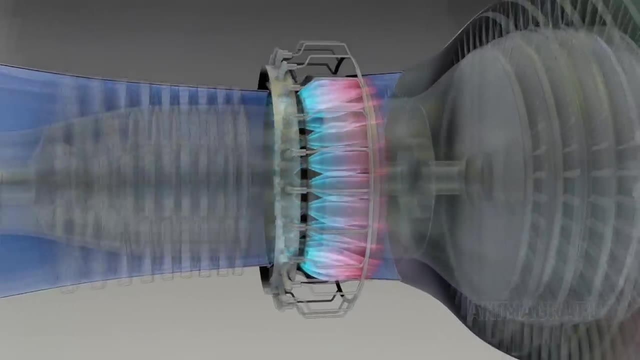 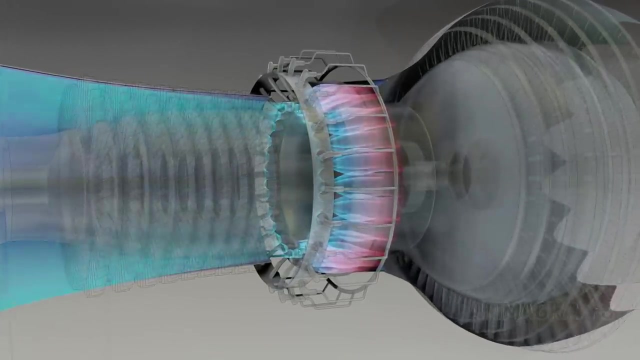 A couple of igniter plugs- not unlike the spark plugs found in car engines- ignite this mixture and the reaction spreads evenly around the ring. The Compostor Once started, combustion continues as long as air and fuel are supplied. The Turbine: 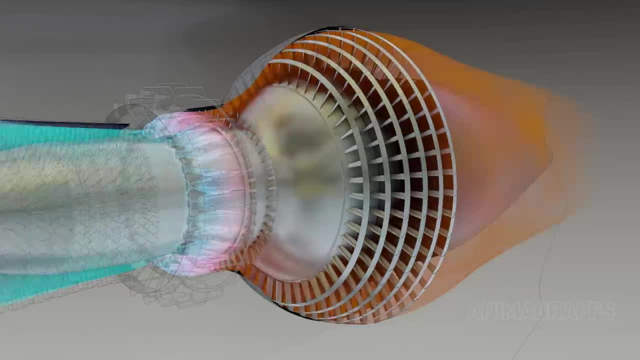 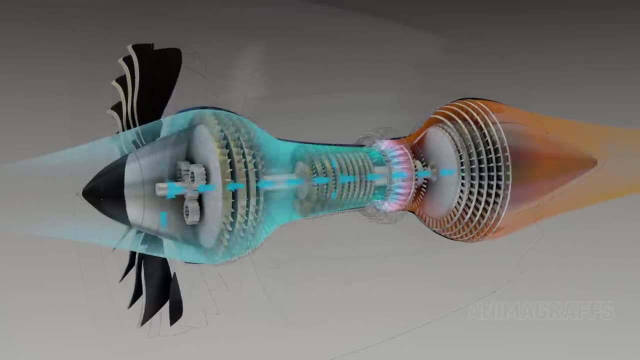 Turbines at the rear of the jet engine are powered by exhaust gases exiting the combustor. Much of the turbine power is used to turn the fan, while a smaller percentage powers the compressor stages. Turbine fins get extremely hot. Some air from the compressor is diverted for cooling. 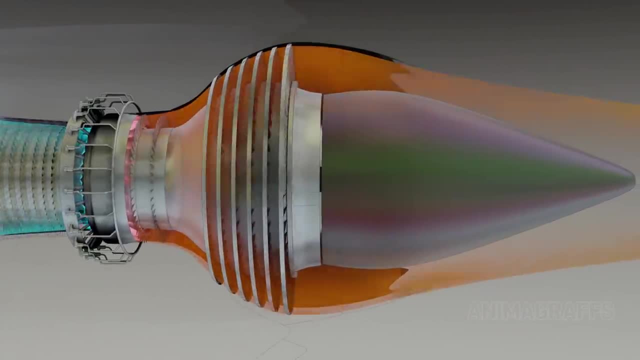 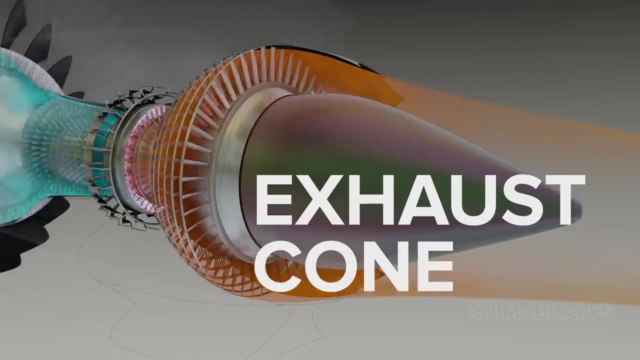 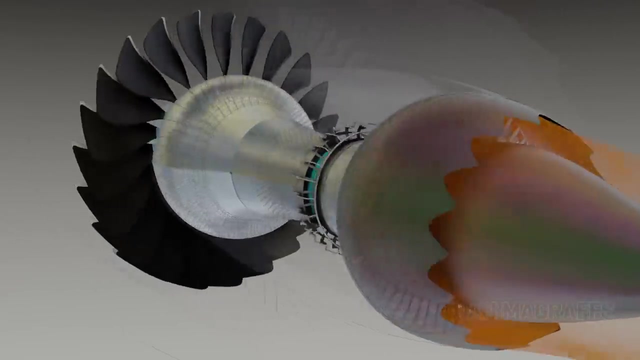 The turbine fins get extremely hot. Some air from the compressor is diverted for cooling And special coatings are used to keep temperatures down. The exhaust cone is specially shaped to mix and accelerate exhaust streams. It also covers sensitive internal engine parts: The Fan. Early jet engines were turbo jets where all incoming air flows through the core. Most modern winged aircraft engines are turbo fans. Most modern winged aircraft engines are turbo fans Where a fraction of air enters the core and the resulting power turns a specially designed 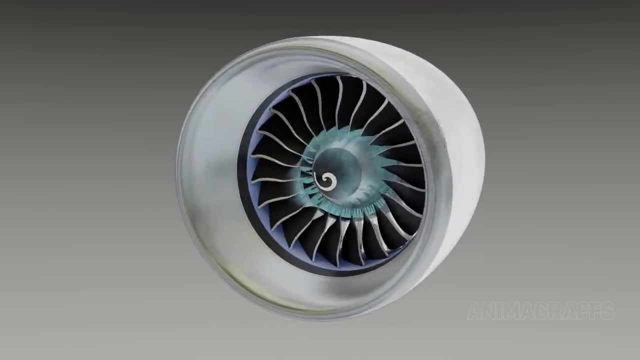 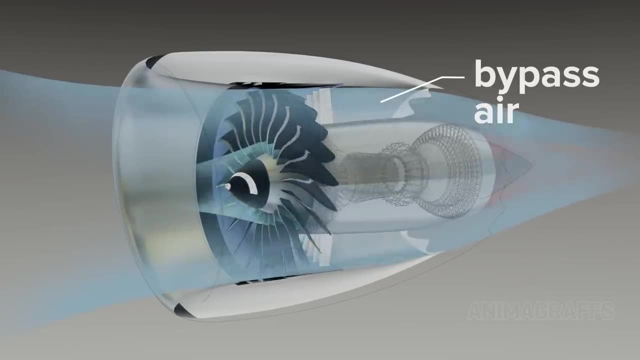 fan. Most modern winged aircraft engines are turbo fans. The fan can be thought of as a high-tech propeller inside a duct. Air that does not enter the core is called bypass air. High bypass engines are designed to move large quantities of air at slower cruising speeds. 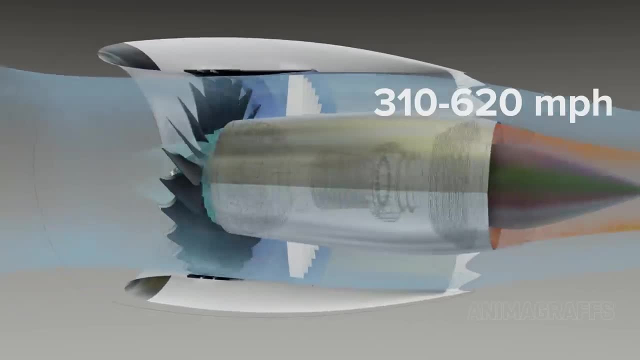 a range of about 310-620 miles per hour. The exhaust cone is designed to be able to move large quantities of air at a slower cruising speed- a range of about 310-620 miles per hour. The exchange for high efficiency is engine size.